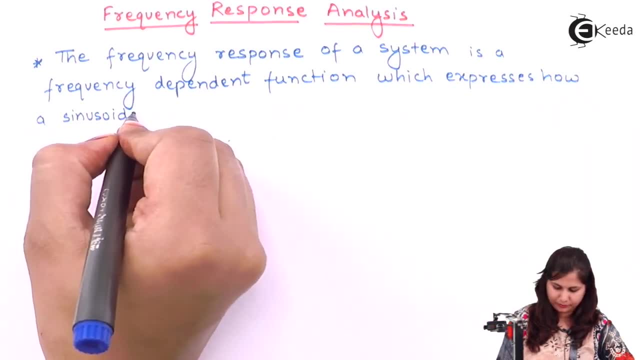 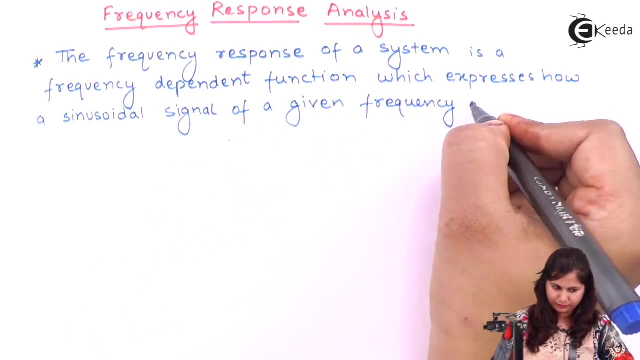 So let's go through the arguments, If we get the question. your answer to that question here is k. it has loads of airport flags, airport masks, airport lights, airport permanents. everything is lightly colored. Pay attention here. I want to show you the errors in a little bit. You're going to see every time we get thoughts. 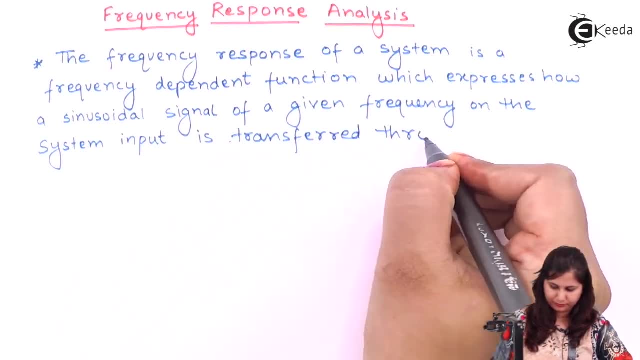 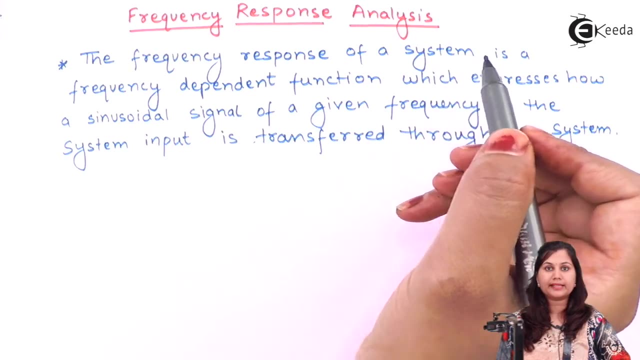 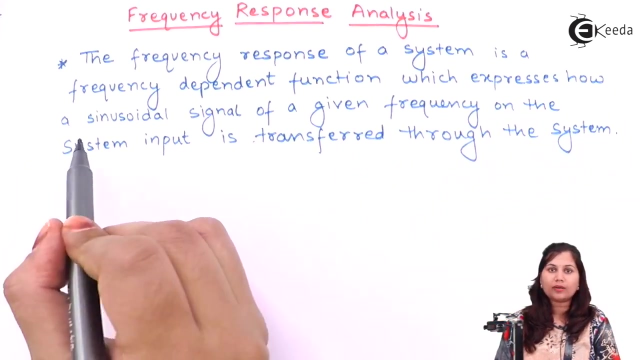 about failure. Did you all get them, Did you? So we're going to find out where you learned. so the frequency response of a system is defined as a free. it is a frequency dependent function which expresses how a sinusoidal signal of a given frequency which is applied on the system. 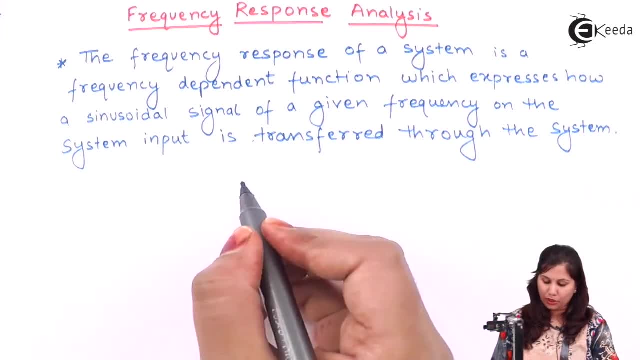 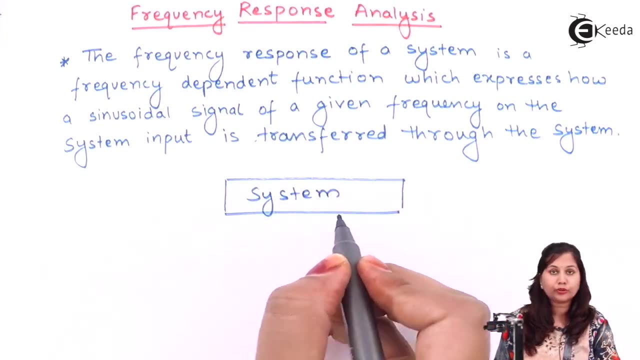 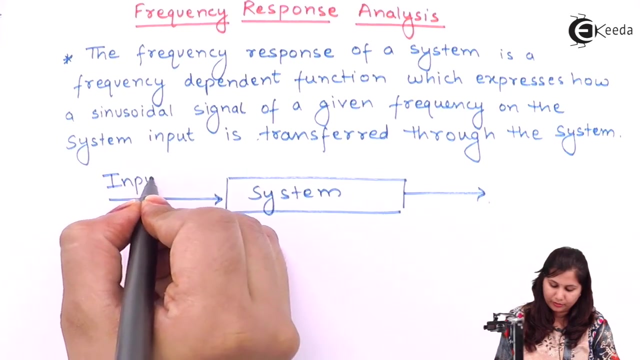 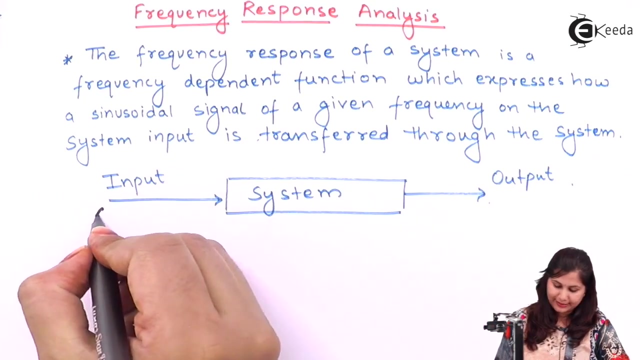 input is transferred through the system. so this is a system, and to the system we apply an input and then we get an output. so this is our input and it is the output. now, input, it is also known as the excitation and output of theásha. 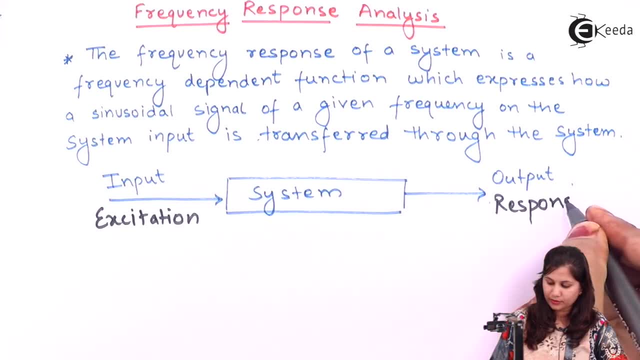 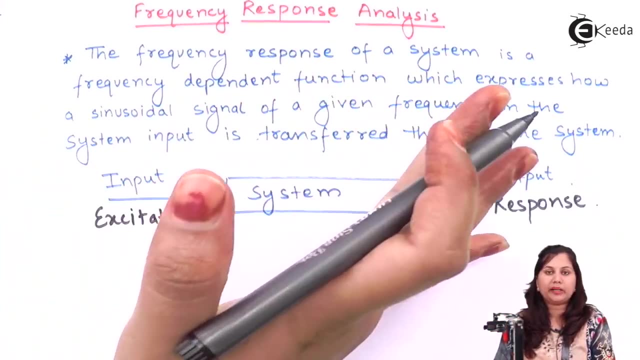 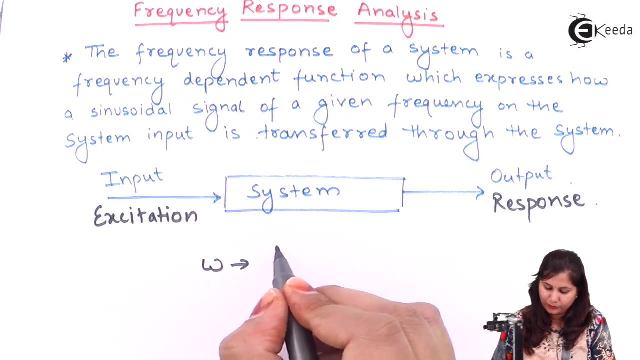 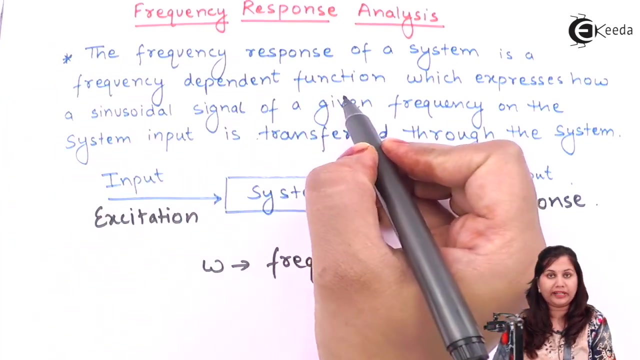 is also known as the response. so for frequency response analysis, the frequency response is a frequency dependent function. so what? on what? it depends on the frequency, that is Omega. Omega is the frequency, so this frequency response will be a frequency dependent function. and it expressed that how a 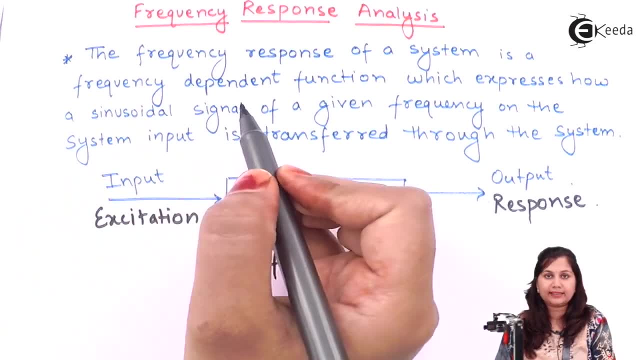 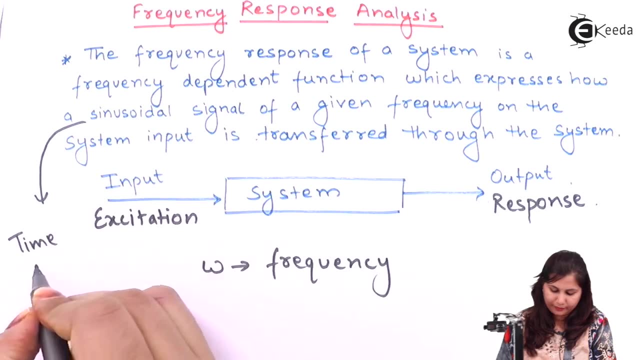 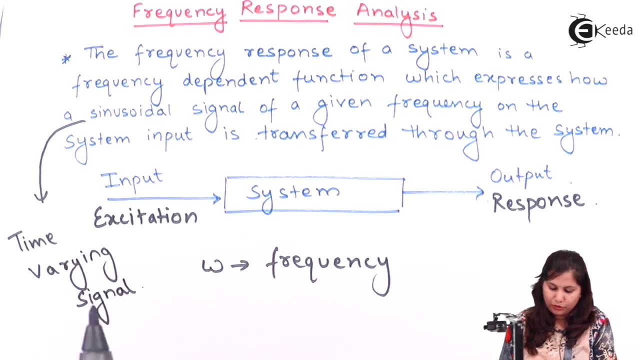 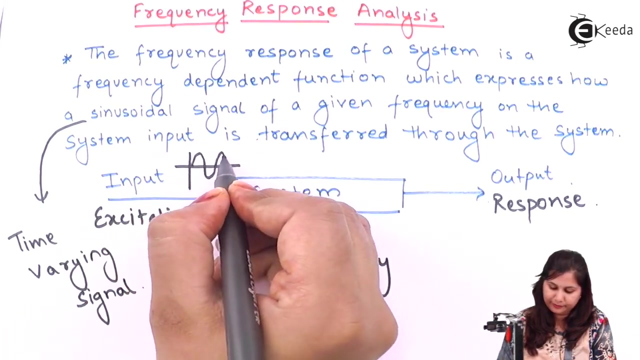 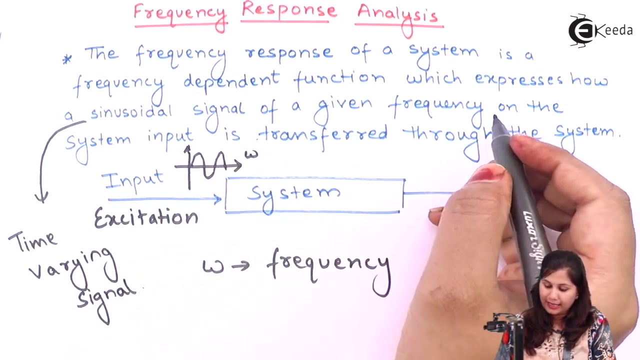 sinusoidal signal. now, this sinusoidal signal, it is a time varying signal. so this input are that? or we can say the excitation, it is a sinusoidal signal and this sinusoidal signal of a given frequency, let us say, suppose omega, and it is given as a system input. and how this input, it is transferred through the. 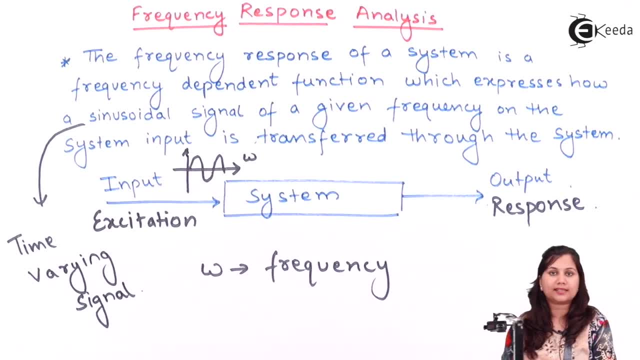 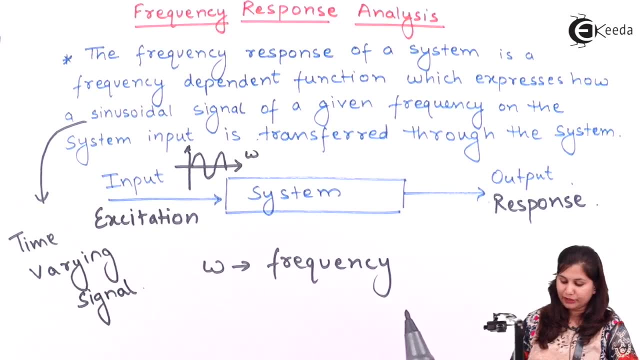 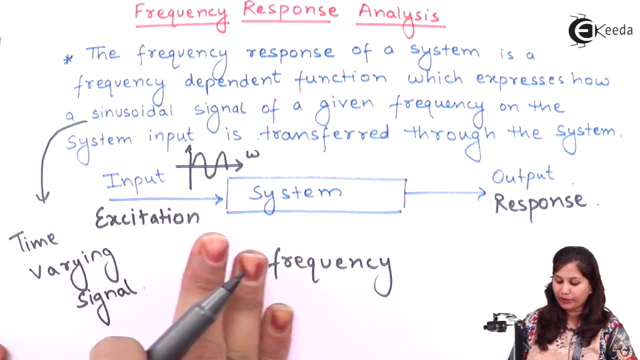 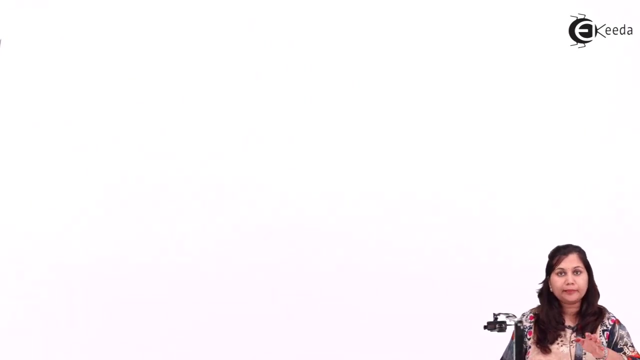 system. it is known as the frequency response of a system. So it is the definition of the frequency response that it is a frequency dependent function. that is omega, which express that how a sinusoidal signal is going to be transferred through the system. Now the input, as we have said that it is 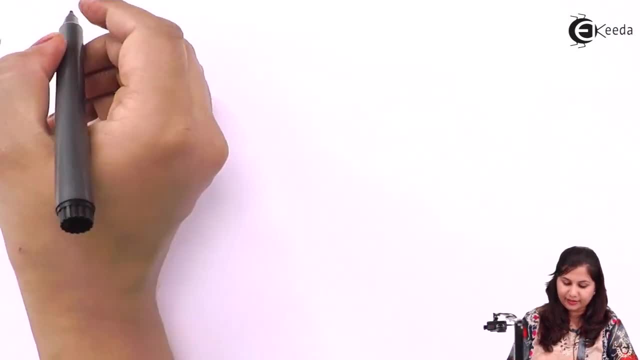 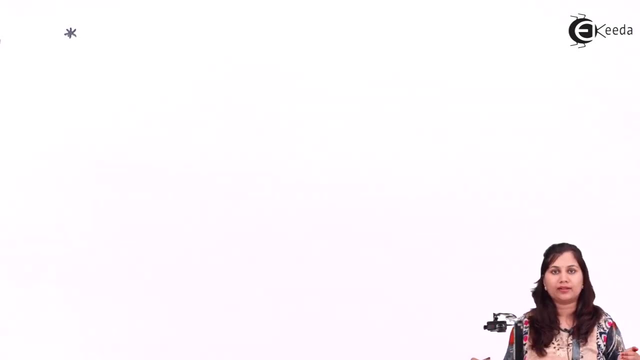 a sinusoidal signal, so it will be a time varying signals. and these time varying signals, they can be considered as a sum of components. When we take Fourier series or Fourier expansion of this sinusoidal signal, then we will see that it is composed of various components and each of this component, it is a frequency dependent function. 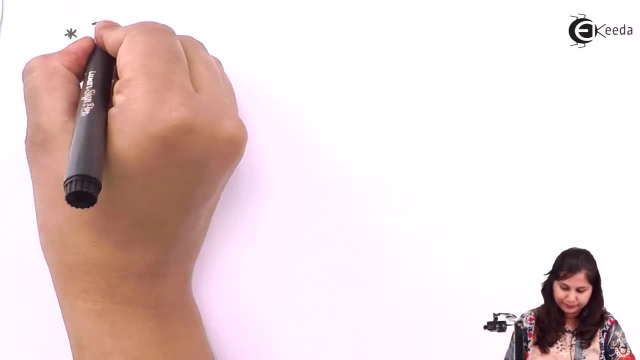 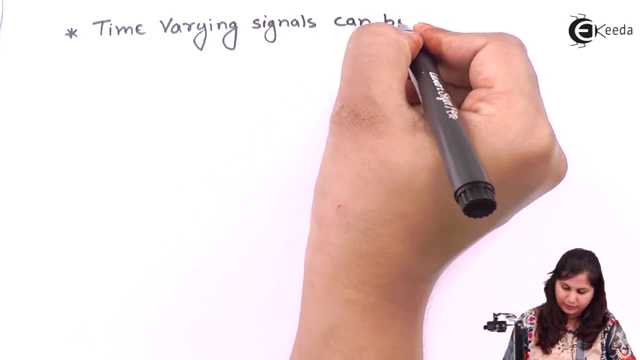 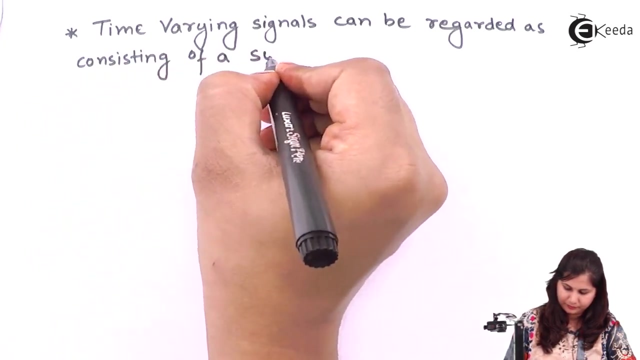 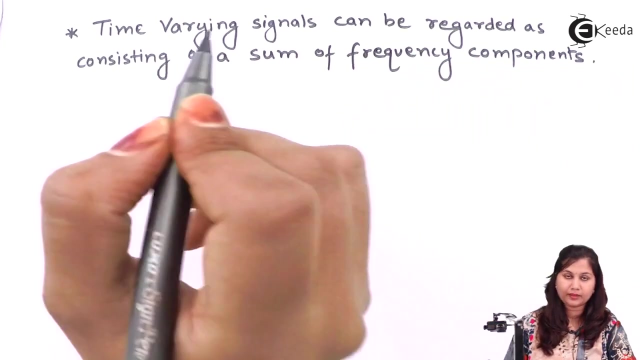 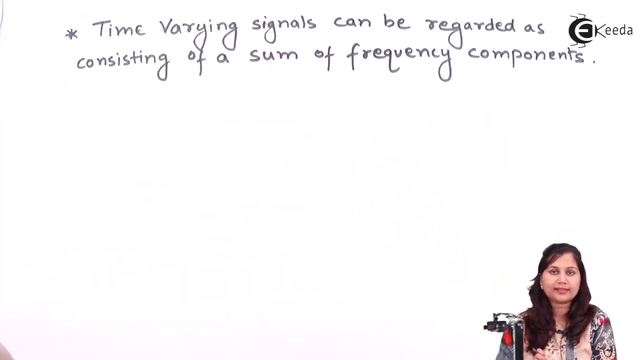 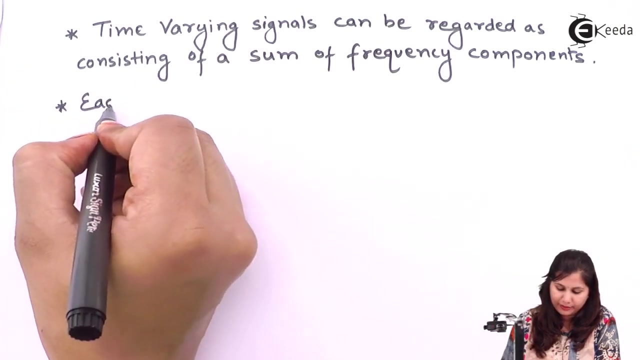 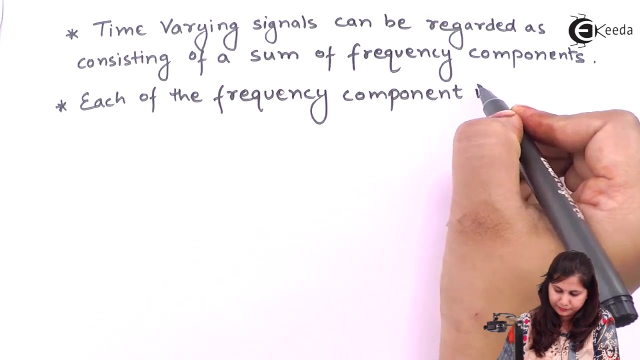 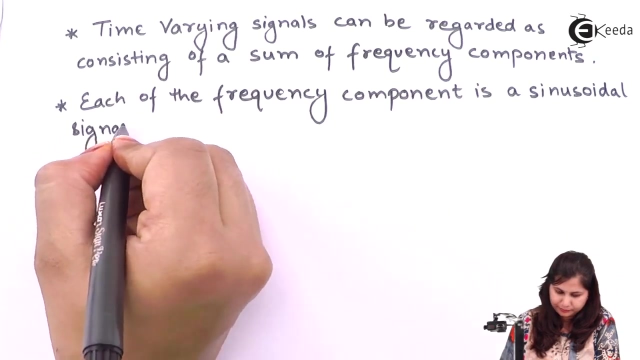 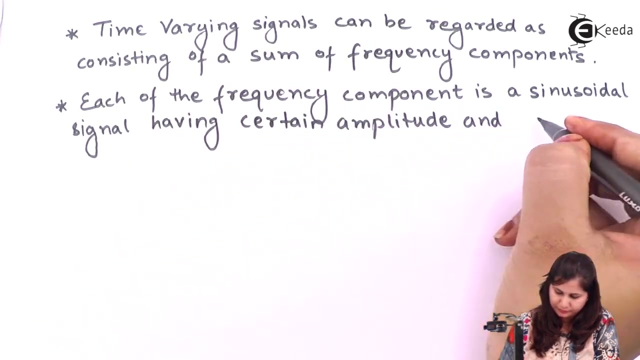 So the time varying signals can be considered as consisting of sum of frequency components. So one signal it will be a sum of various frequency components and each of these frequency component is a sinusoidal signal that have a certain amplitude and a certain frequency. So a time varying signal. 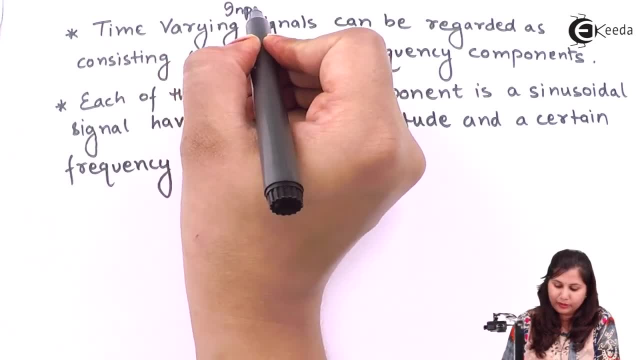 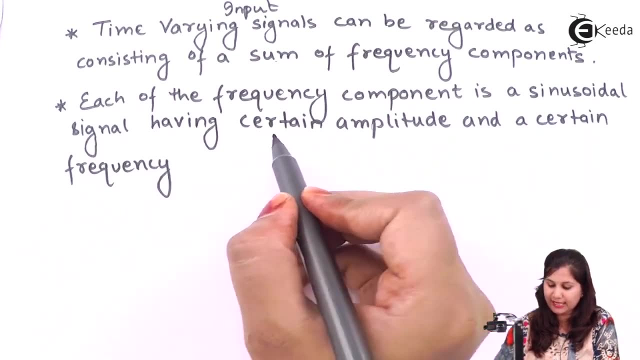 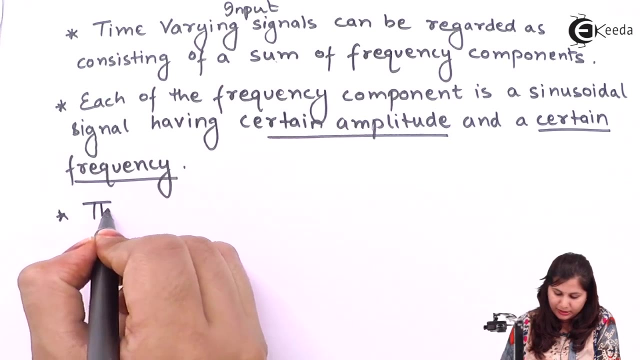 So a time varying signal, that is an input. it will be a sum of frequency components and each of the frequency component is a sinusoidal signal which is having certain amplitude and a certain frequency. okay, Now the frequency response. we have to classify it and we are going to say that the frequency response. 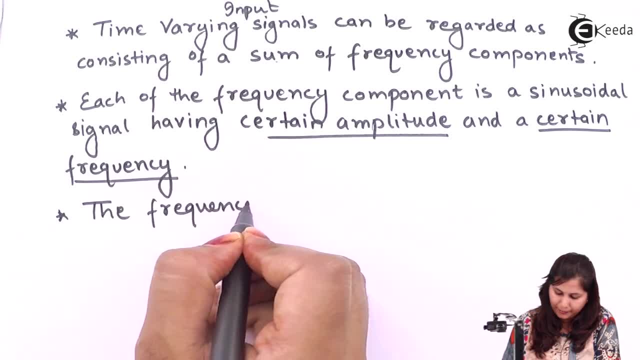 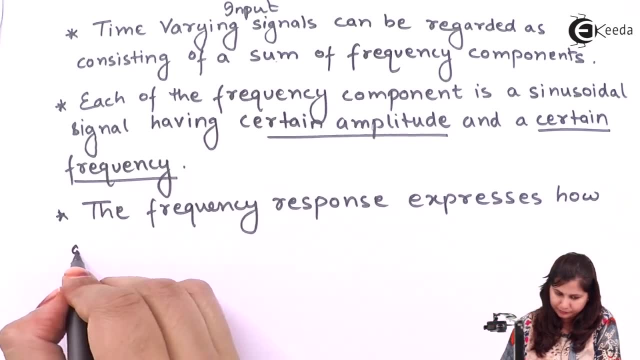 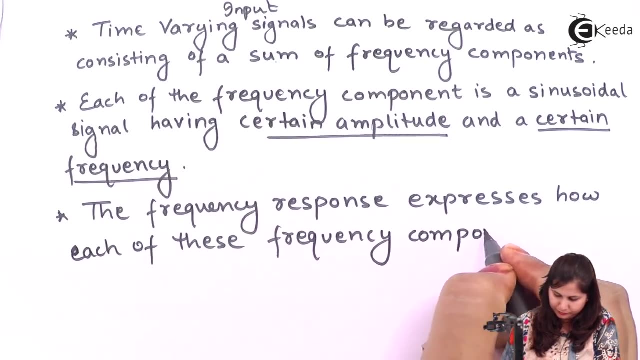 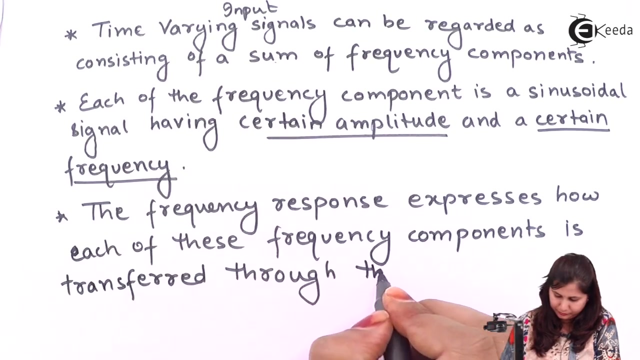 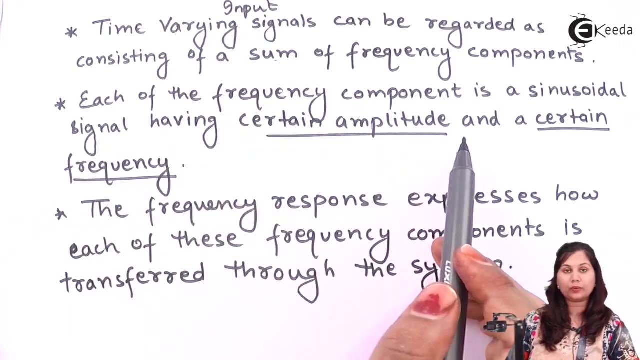 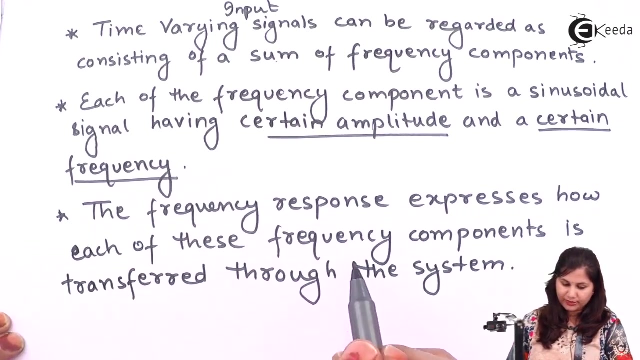 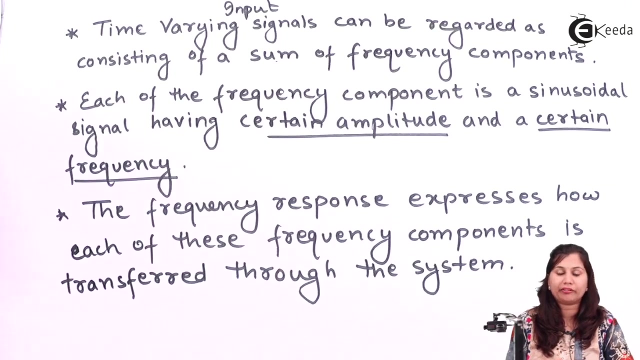 what it does. now the frequency response. it expressed that how each of these frequency component it is transferred through the system. okay, so these out of these frequency components. it may be possible that some of the frequency components they are attenuated or they can be modified or some noise can be introduced. 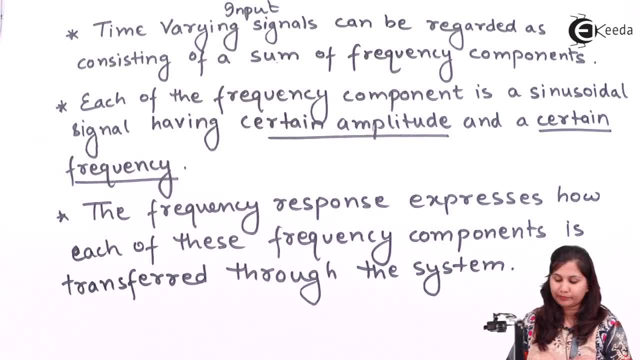 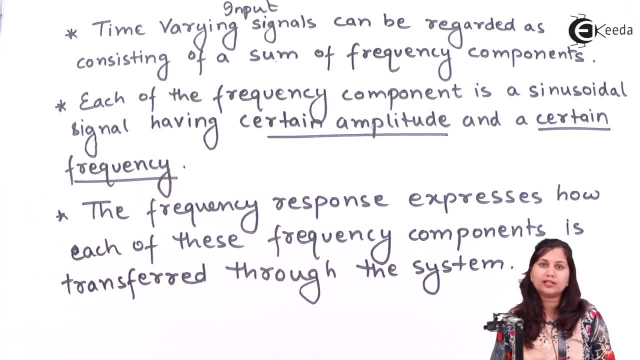 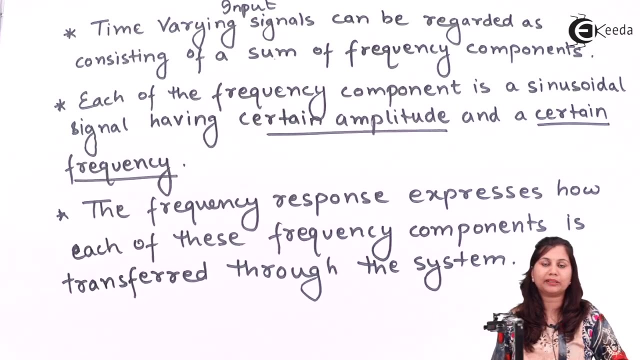 or there can be some phase difference. there may be some modifications which can be caused. when this these frequency components, they pass through the system, so the output which we will get it will be something different, because some modifications has been done while these frequency components are transferred through the system. so some 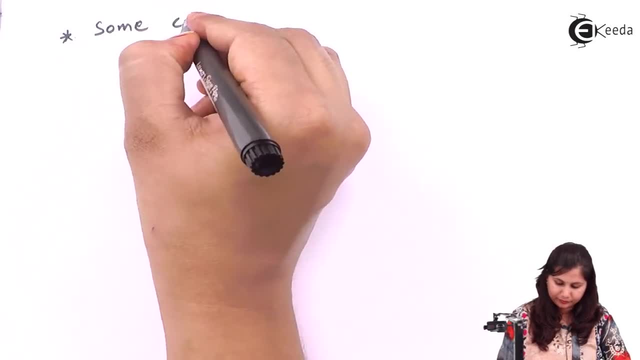 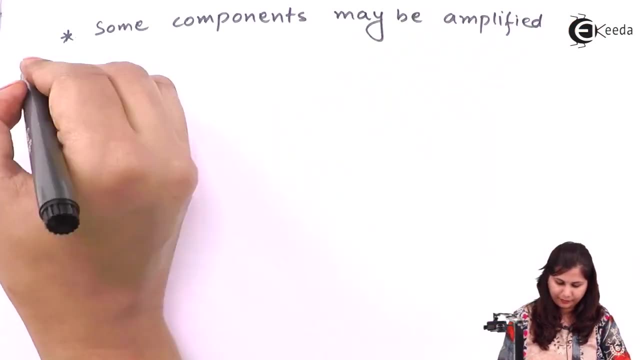 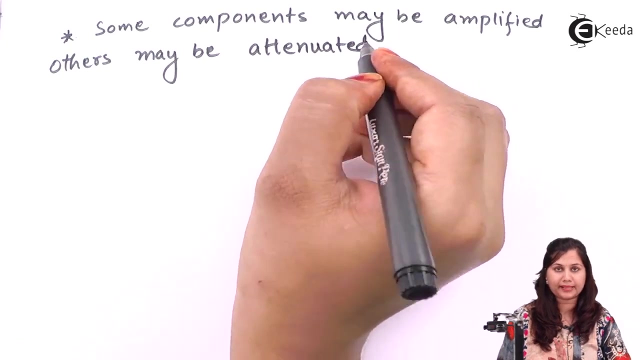 of the components. they may be amplified, others may be attenuated. attenuated means they are suppressed- okay, attenuated, and there will be some phase lag through the system. okay, so what this frequency response is doing? it is transferring a cycle between a sil- Behaviorhip response to absorption- and Intuition System. 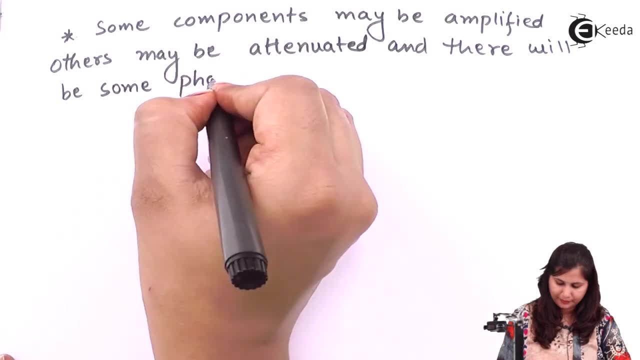 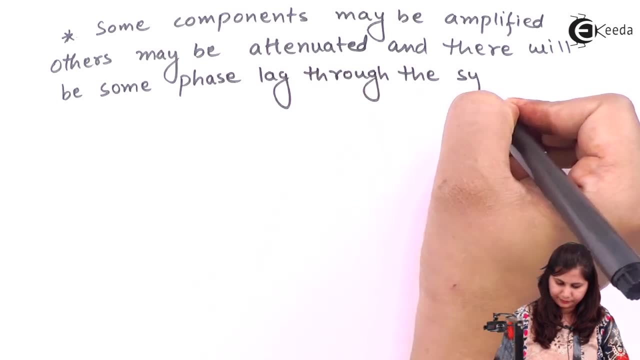 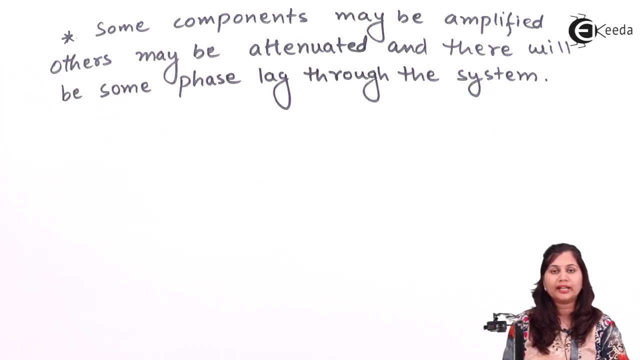 atten Huge dynamic log, they are suppressed. okay, so what this frequency response is doing? it is transferring a cycle betweenvas, a frequency response, to absorption and Intuition System signal, and this sinusoidal signal is applied on the system input and then it is passed through the system. so the frequency response is expressing that. 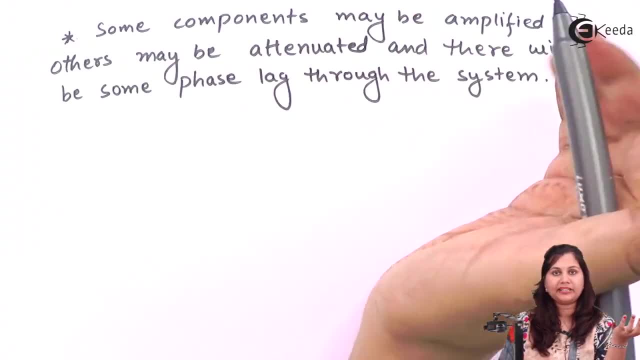 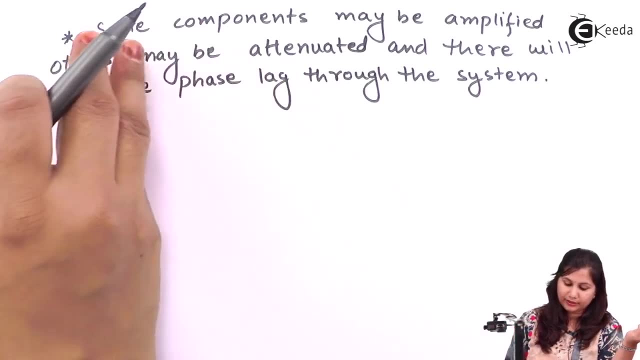 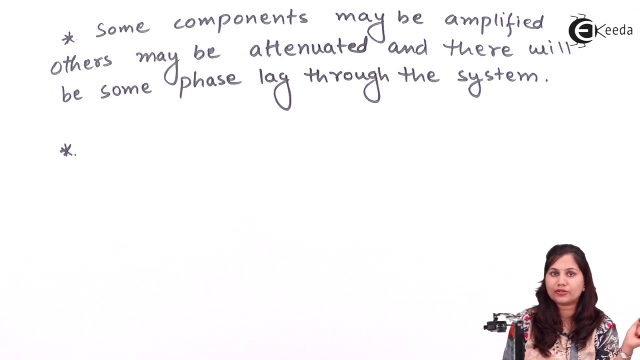 how this is transferred, whether it is amplified, whether it is attenuated, or is there any phase difference in this signal? so this frequency response, it can be used in the analysis and the design of the control systems because it is showing us that how the time varying signals is passed through the system. so 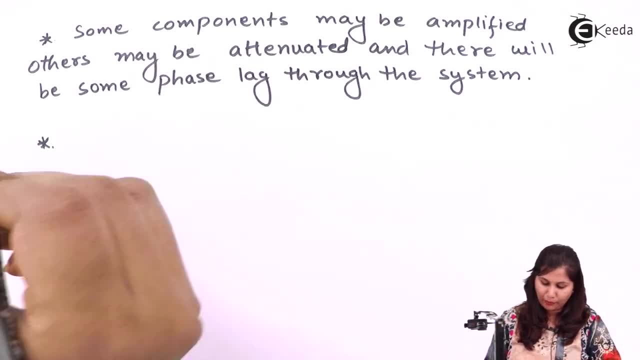 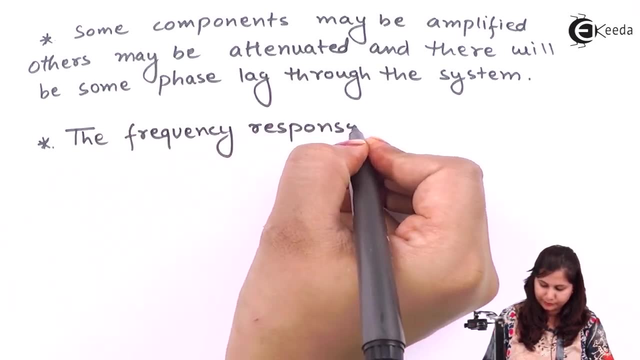 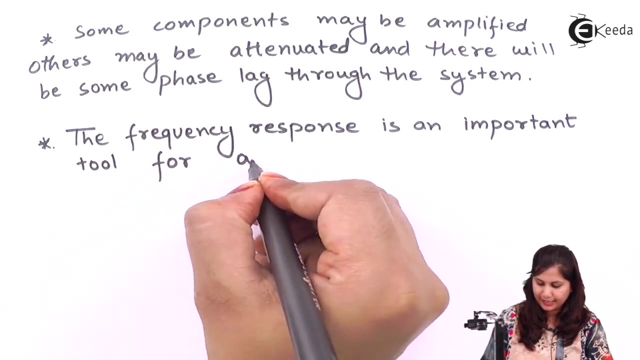 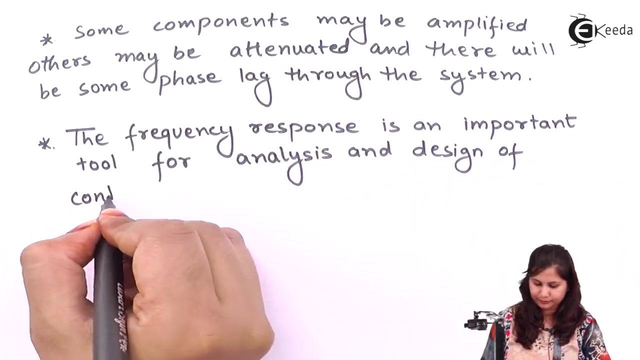 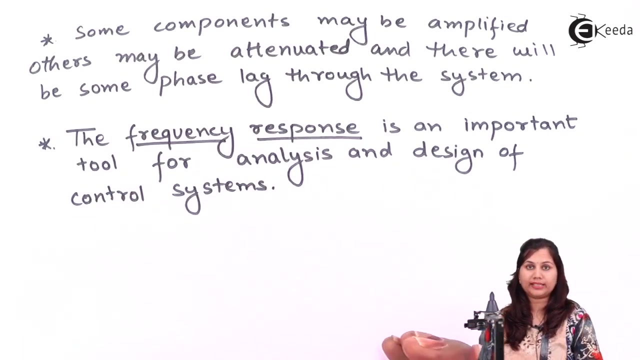 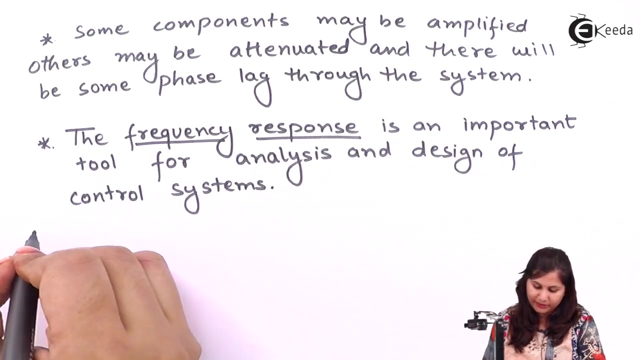 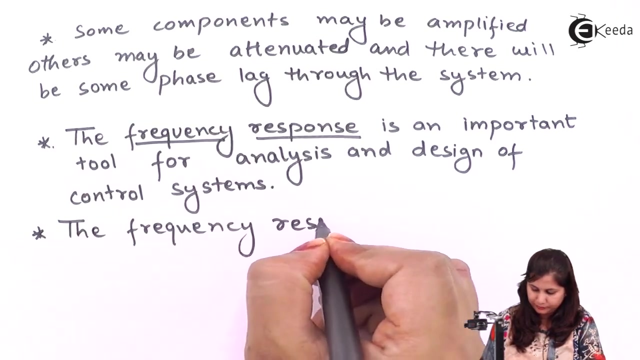 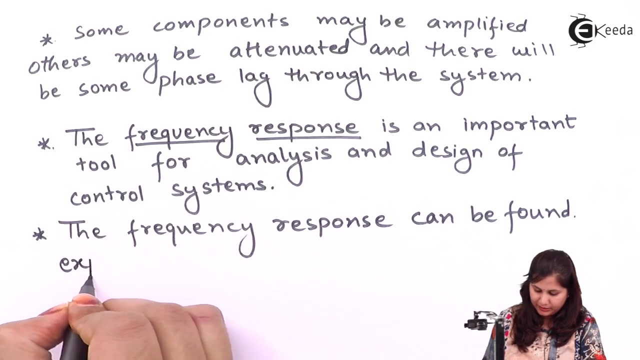 the frequency response. it is an important tool for analysis and design of control systems. so this frequency response is, it is playing an important role. it is very important for the analysis and design of control systems. so how we can obtain this frequency response? the frequency response can be determined. it can be found experimentally or from the 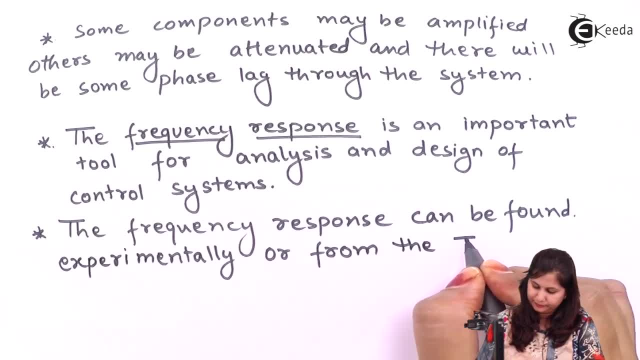 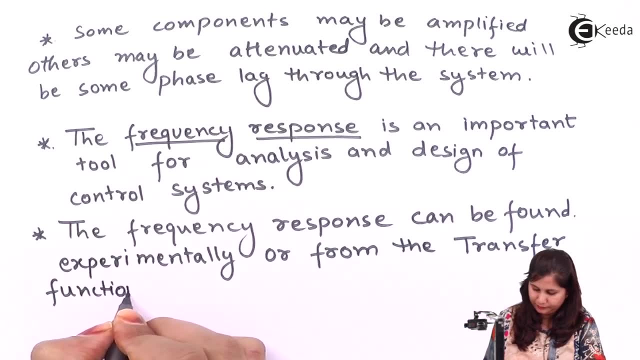 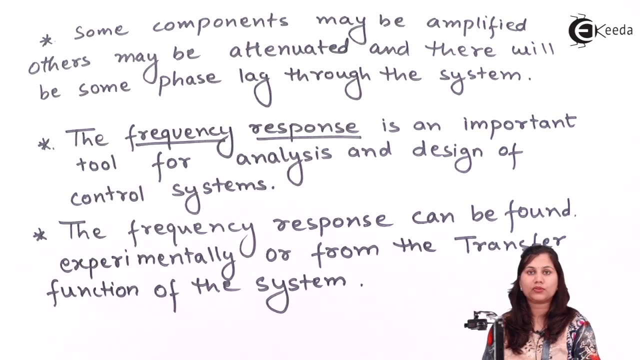 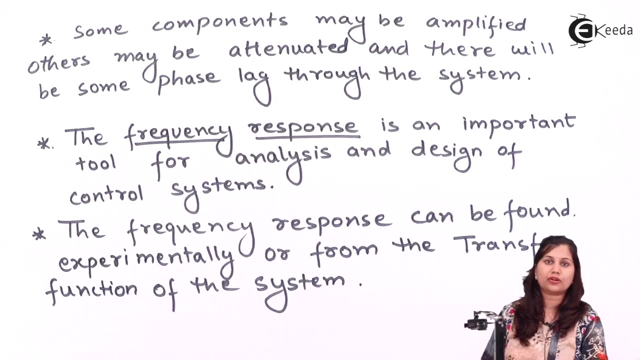 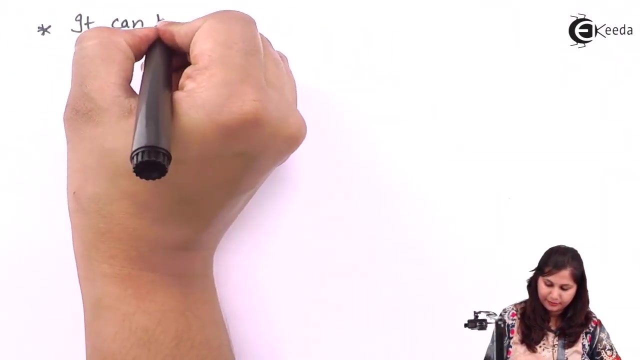 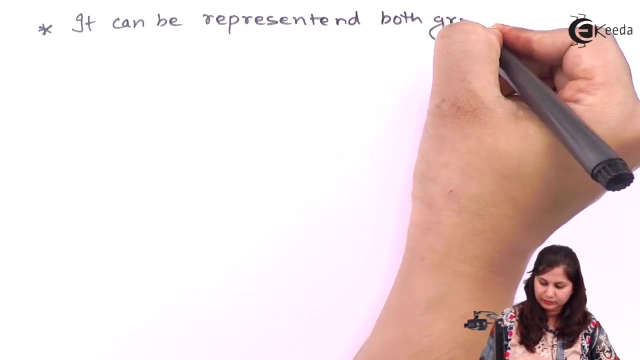 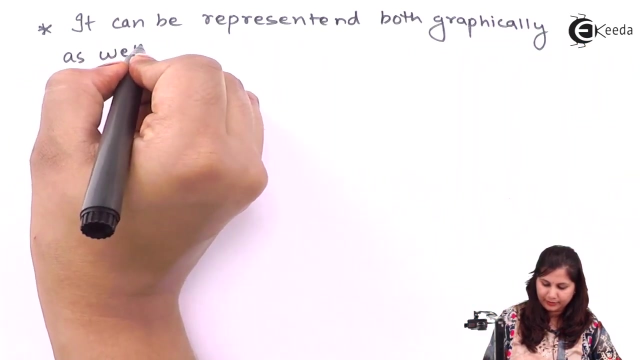 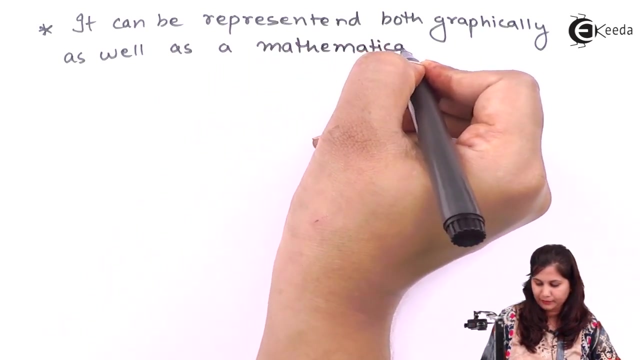 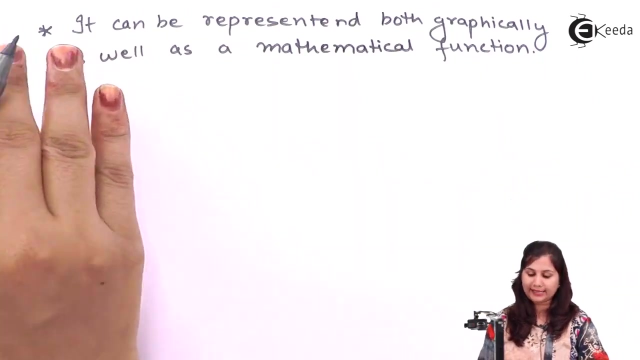 transfer function of the system. so we can find out the frequency response of a system by some experiments, or we can obtain it from the transfer function of the system, and it can be represented both graphically as well as a mathematical function. So you can express the frequency response of a system graphically also. and 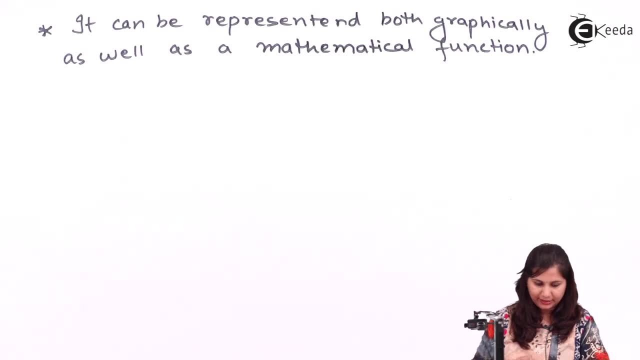 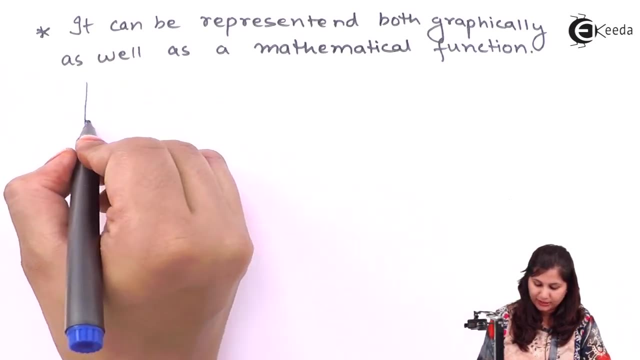 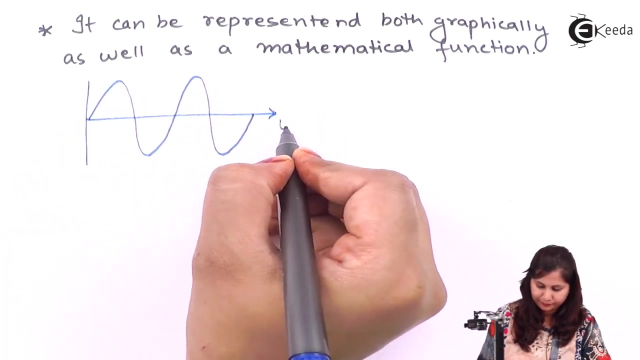 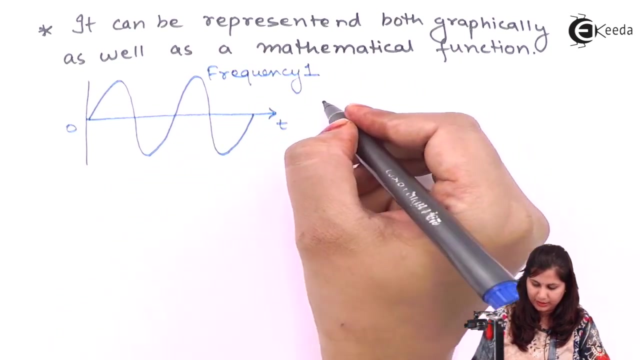 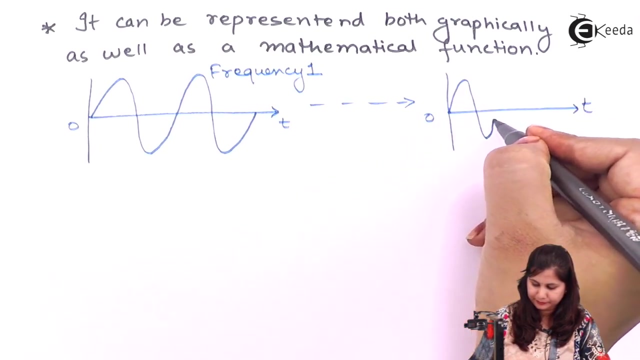 as a mathematical function also. so if we see that we were having an input, a enabled Okey, a sinusoidal function, and it is composed of water, Therefore water is generated. frequency components. and suppose this is a frequency component, this is at frequency. suppose it is first frequency and we are getting the output as okay. 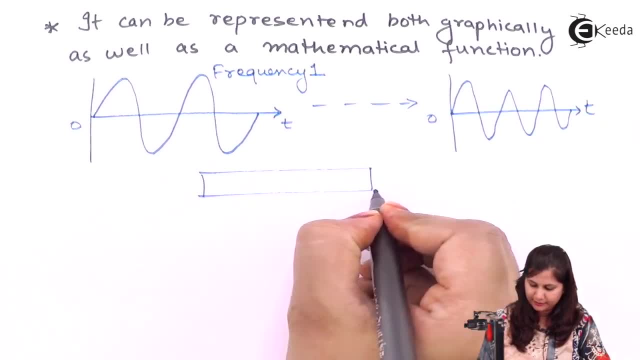 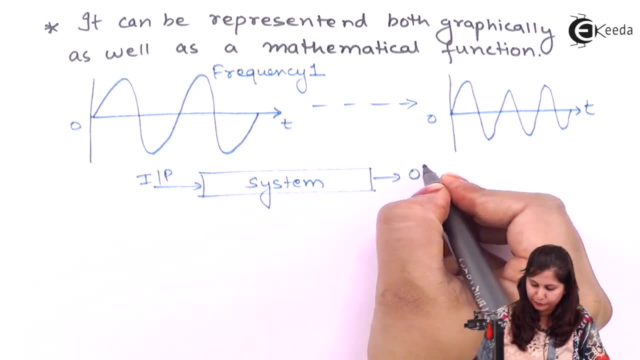 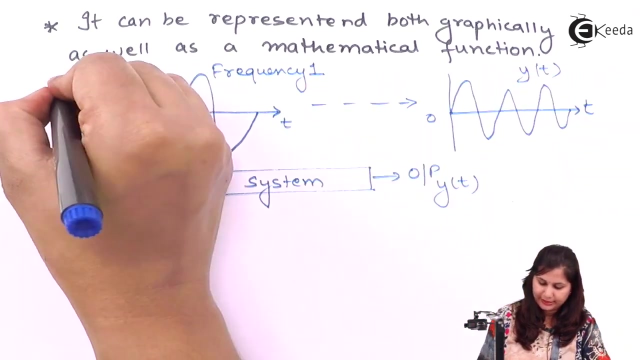 this is our output. so this is the system and on the system we are applying the input and getting an output. input is XT and this is YT. so this is our YT output and this is our input XT, and it is on one frequency. now for second frequency. 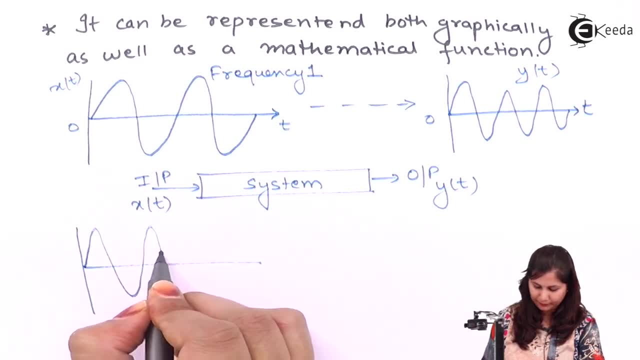 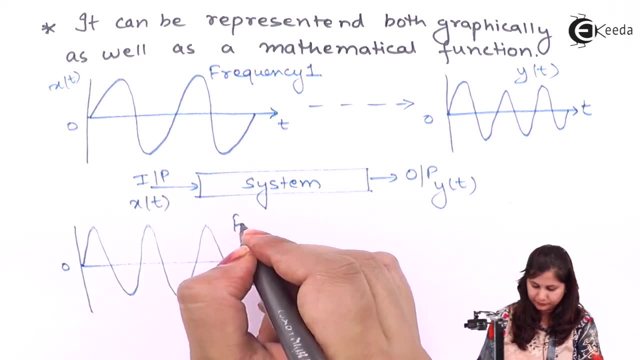 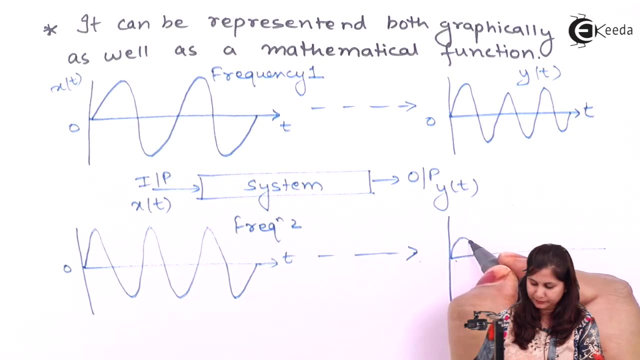 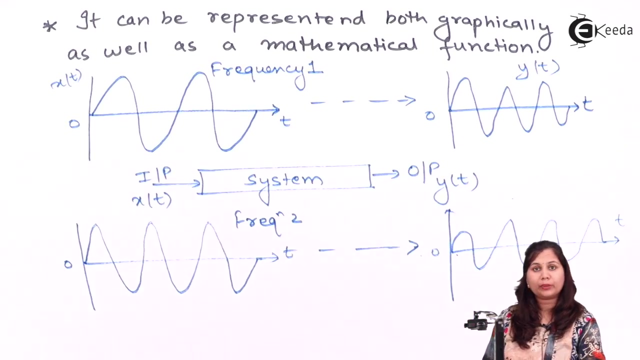 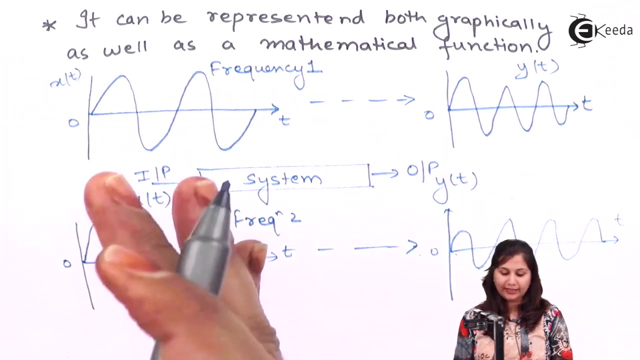 the output may be different. this is frequency. second, and for this we are having some different output. so frequency response is telling us that at what frequency frequency is different and depending upon the frequency, what is the output. so our output will be a function F. I can a gave a function that is given to us, the input is going to be: